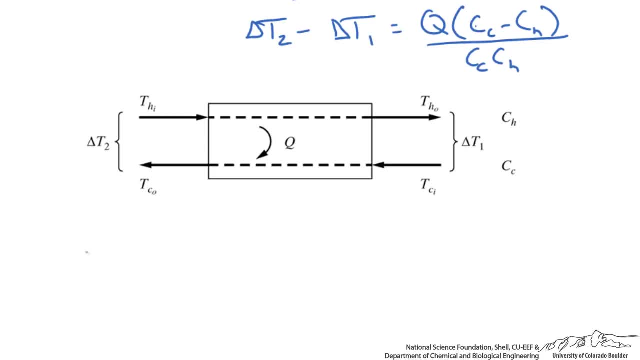 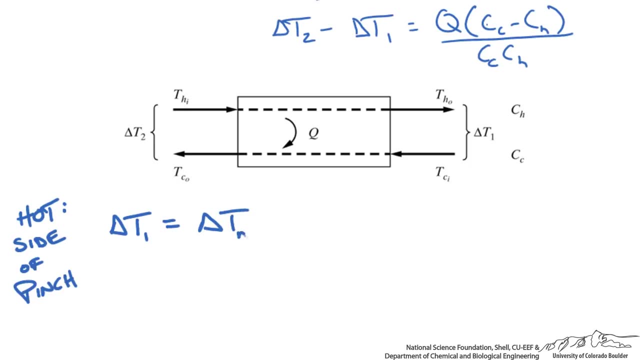 them in the following manner. First, we use this equation and say that if we're designing on the hot side, then delta T1, this is for the hot side of the pinch- delta T1 is going to be our designated minimum approach temperature. This leaves us with a delta T2 equaling delta. 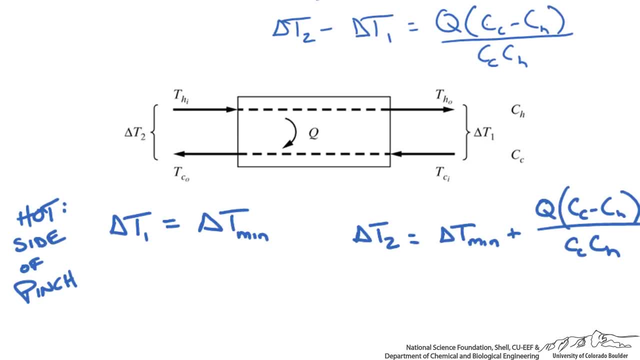 Tmin plus the value on the right side. Now, to make sure that our delta T2 here is going to be greater than our approach temperature, this value on the right side has to be positive. Now Q is positive and our heat capacity flow rates are positive. That means CC has to be greater than or equal to CH. Now the following: 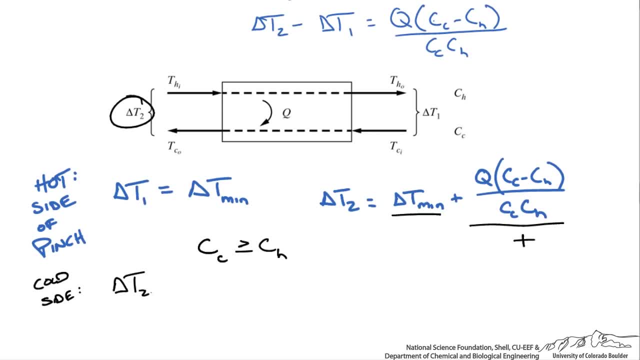 is going to be true. if we're looking at the cold side, We set delta T2 equal to delta Tmin. We rework this equation. This time there's going to be a negative, So we're going to get a negative sign. Now for this to be true and make sure that our delta T1 is greater. 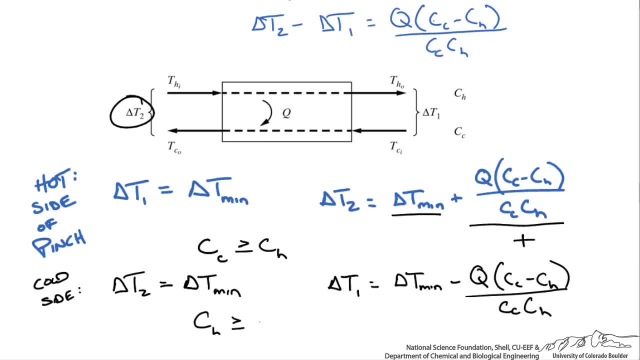 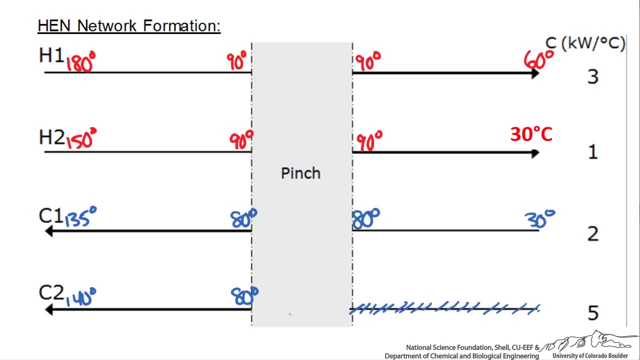 than delta Tmin. our CH has to be greater than or equal to our CC. So we use these two guidelines when we're designing our heat exchanger networks to match streams and determine whether or not it's a feasible match. So let's practice this on our diagram here, where we have our 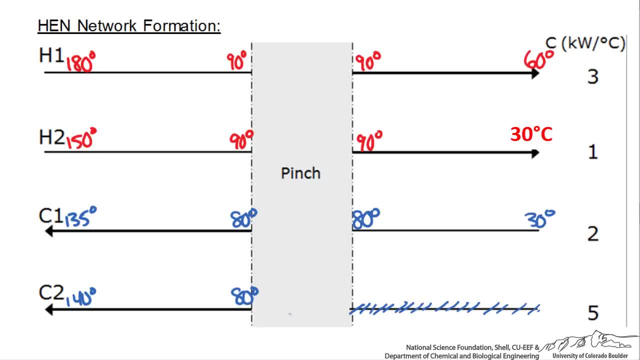 four streams: our pinch point, our pinch temperature for both the hot and cold stream, and our source and target temperature. If we start with the hot side, which is arbitrary, but something that is typically done is to start with the hot side of the pinch, Then we want to match two streams such that the 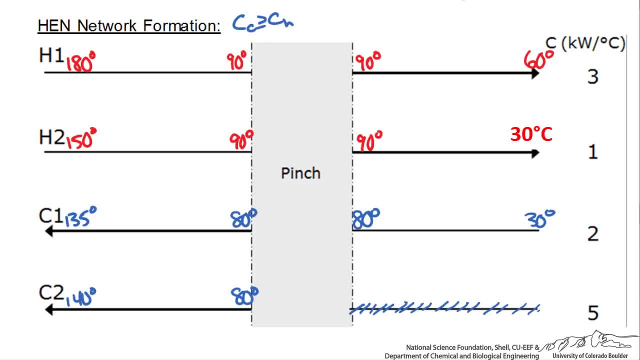 CC is greater than or equal to CH. So in that case, if we matched C2, we can match it with either H2 or we can match it with H1, since in both cases our value of 5 is greater than the values of the hot streams. 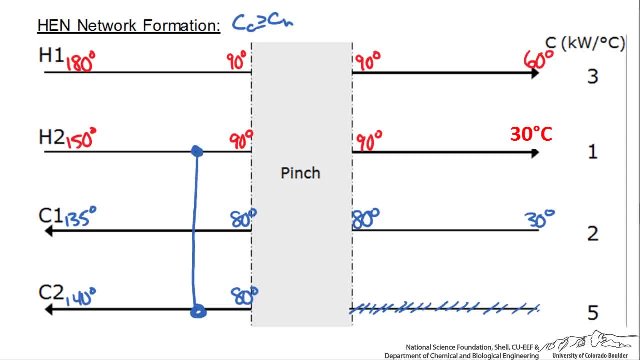 However, if we match C2 with H2, and try to match C1 with H1,, you would see that H1 has a higher specific heat flow rate value than the cold stream, and that would mean that the stream match is an infeasible match. So we wouldn't want to do that, but at least let's start with. 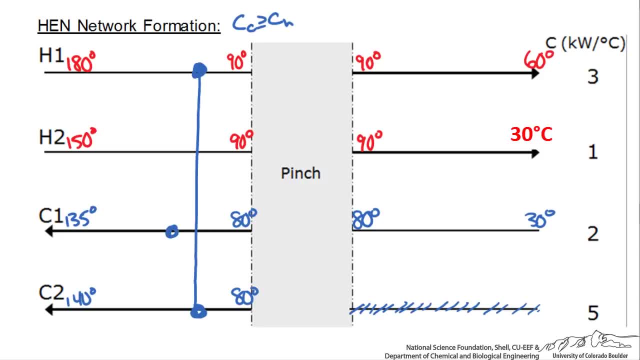 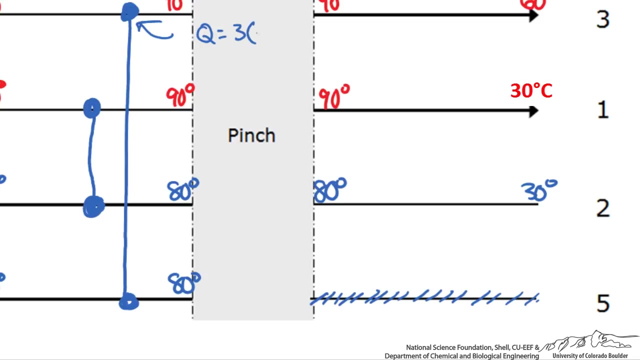 C2 to H1, and then also draw C1 to H2.. So we want to do this to maximize the potential load on the heat exchanger. so we would calculate what the heat transfer would be for that connection. So if we look at this node right here and we say that Q is equal to 3 times the difference, 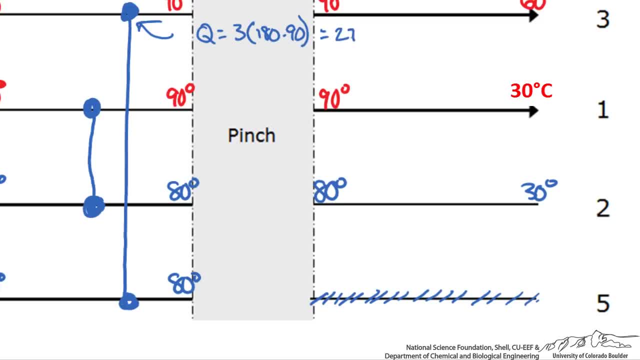 of 180 minus 90, then we would get 270 kilowatts. We do the same thing for the other node and we would see that 5 times 140 kilowatts, So we would get 140 minus 80, is equal to 300 kilowatts. As you can see, at this node we 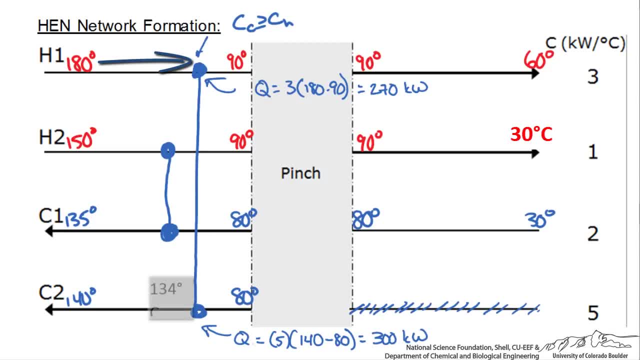 could decrease the temperature from 180 all the way to 90, but we cannot increase the cold stream from 80 to 140.. So we could check mark that node, knowing that we could go from 180 degrees and cool it to 90 degrees. but for the other node, we know that this load. 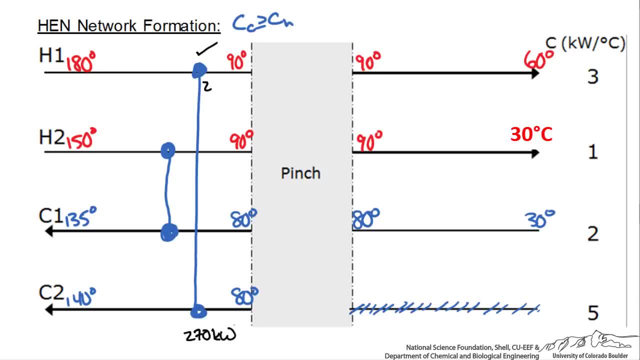 is 270 kilowatts, which means that we could raise the temperature from 80 degrees, and we get that Using the same calculation, just showing that Q is equal to 270 times 5, and the temperature difference, which we could say, is X- some unknown temperature, minus 80.. 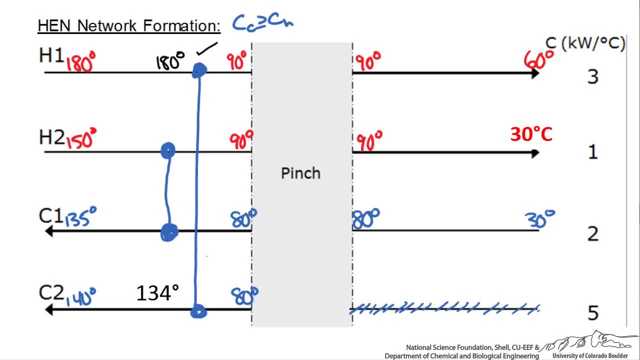 And we could calculate the load from our stream, our connection from H2 to C1. Again, you can see with the hot stream we have a lower load than that with the cold stream. So we can decrease from 150 to 90, but we cannot increase the cold stream 1 from 80 to 135. 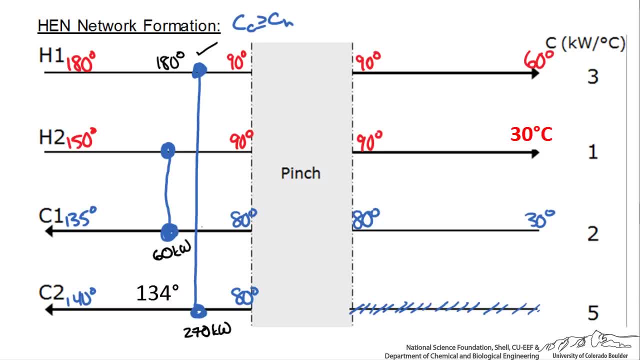 So again we write the load under the connection and we calculate what the new temperature would be, which in this case would be a 30 degree difference and a maximum of 110 degrees. So we've already reduced our hot streams from the inlet to our pinch temperature. so we 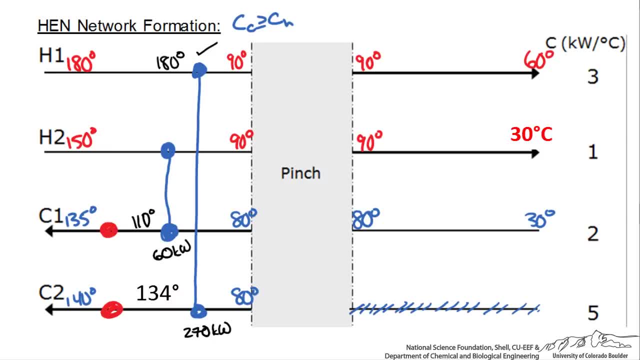 need to add some kind of hot utility to raise it from their temperatures to their final target temperatures And we could write again what the duty on these utilities would be so to go from 110 to 135, change of 25 degrees times our capacity ratio of 2, would give us 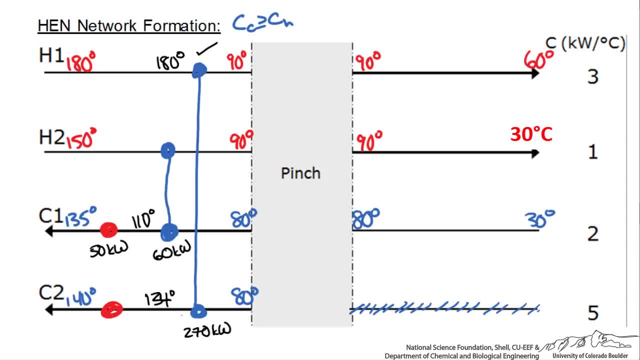 50 kilowatts. So our temperature difference of 6 degrees times our heat capacity flow rate gives us a load of 30 kilowatts for this exchanger. So, as you can see, adding up the exchangers on the left side, we have 80 kilowatts, which 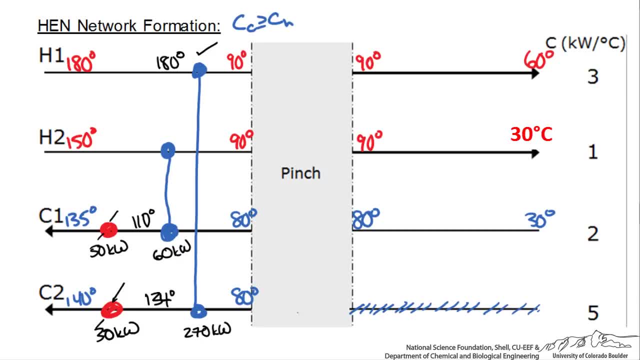 is what we had calculated before as our minimum energy requirement target for the hot stream. Now, moving to the cold side, we do the same thing and we follow the rule that our hot side loads have to be greater than our cold side. So we don't have a C2, we just have the C1 to work with. 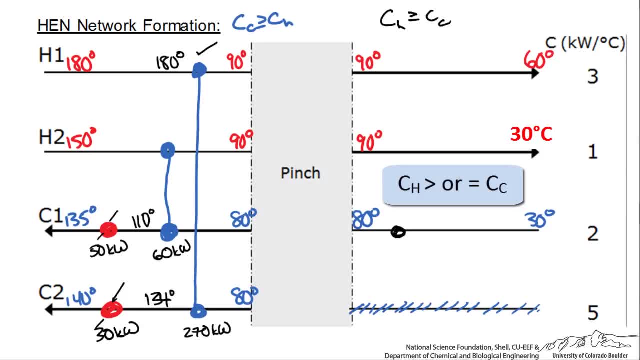 So let's match that, following the rule that it has to be higher, we'll match it with H1, and we'll calculate the Q associated with this. If it were to go from 90 to 60,, that would be a temperature change of 30 times 3,, which. 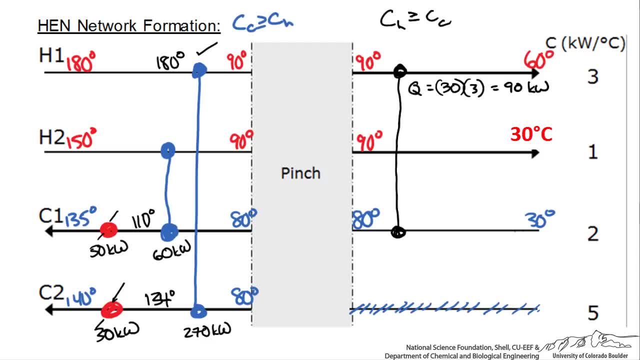 gives us 90. On the bottom, to go from 30 to 80, gives us 100 kilowatts. So again our limit is 90 kilowatts. so we'll put that under the exchange, Calculate what our temperature difference would be, so we could completely cool our. 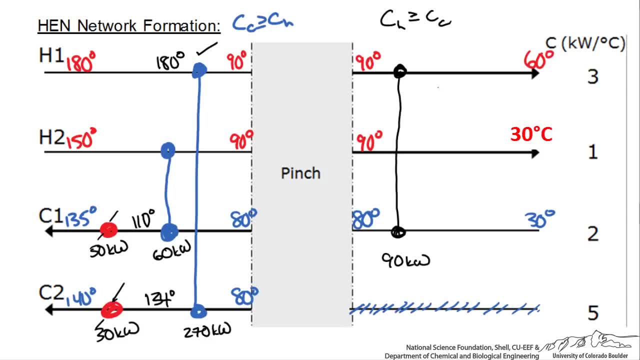 hot stream 1 from 90 to 60, but we can only heat up our cold side stream from 80, and this is going to be 35 degrees. We calculate that again By 90, equaling 2 times 80 minus X, and you'll see that X is equal to 35.. 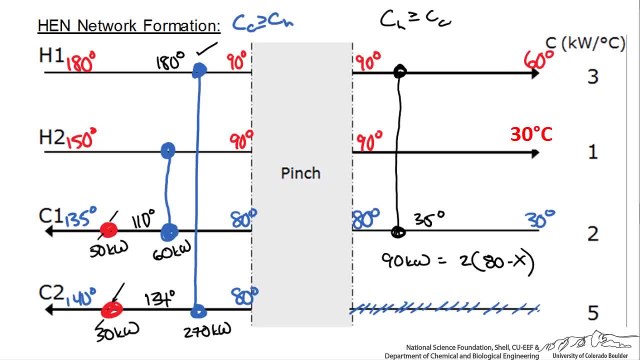 So now we need to cool our H2, and we could either do that trying to use our cold stream or cold utility. Since we're at 30 degrees as our inlet and 35 as our outlet, we're not going to worry about crossing over our minimum approach temperature. 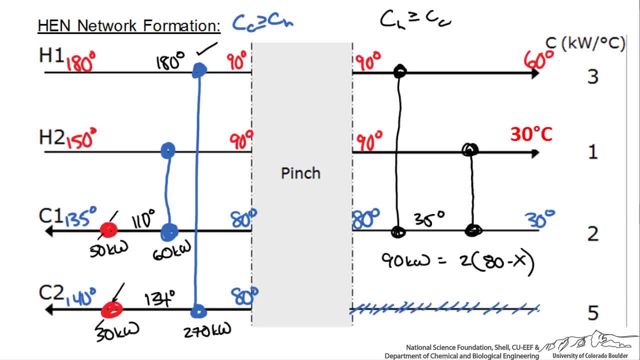 So we could go ahead and try to match these up And the load that we would have would be the 5 degrees times 10, so it would be 10 kilowatts, So we can effectively cool down H2 10 degrees to our 80 degrees Celsius. 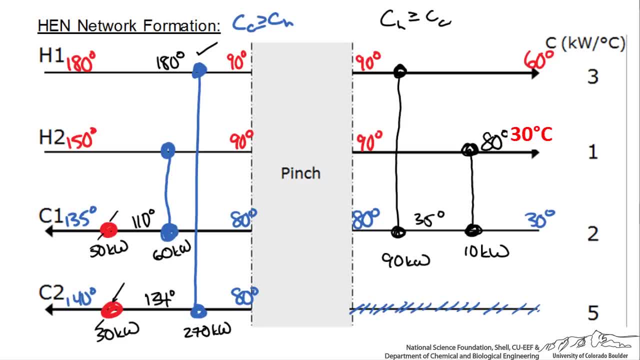 However, our final temperature that we are looking for for our H2 stream is 30 degrees. So at this point, we've completely heated our C1 stream, We've completely cooled our H1 stream and we have to further cool H2, so we have to.